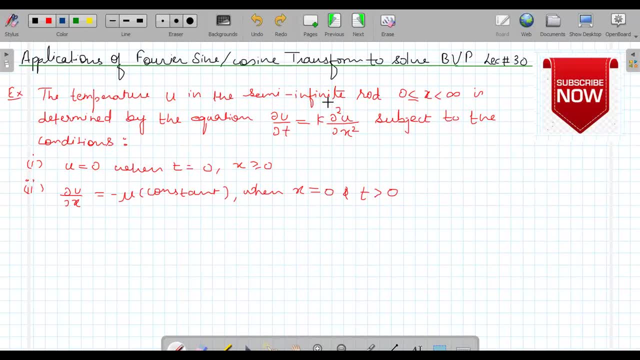 can see. The problem is the temperature u in the semi-infinite rod is determined by equation: del u by del t is equal to k. del 2 u over del x square, Subject to the condition u is equal to 0 when t is equal to 0.. x is greater than or equal to 0.. And del u by del. 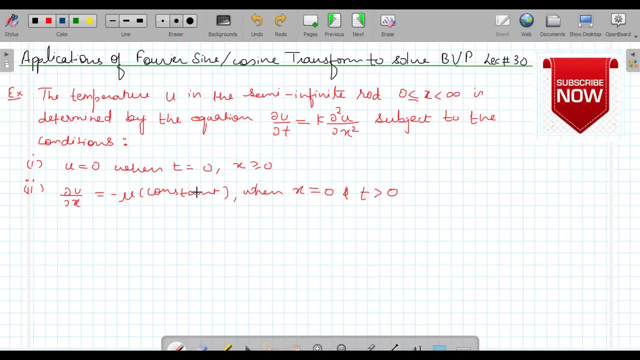 x is equal to 0. And del t is equal to minus mu, where mu is a constant, when x is equal to 0 and t is greater than 0. That means the meaning of first condition is that the temperature is 0 when time is. 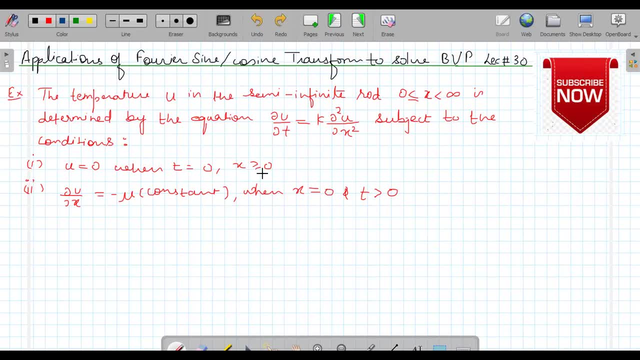 0. And x is greater than or equal to 0 means initially the temperature is 0 in the rod. Okay, And the meaning of second condition is that del u by del x is equal to minus mu when x is equal to 0 and t is greater than. 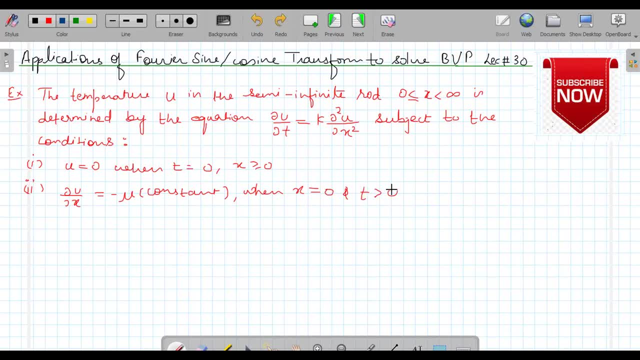 0 means as you increase the time, x is equal to 0. means at the end, at the boundary of the rod, the temperature rate of change of temperature is minus mu, which is constant. the temperature is constant at the initial. just say a rod here. if you have this rod, 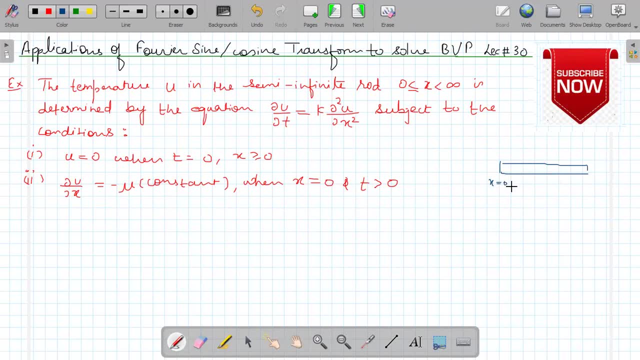 and this denotes x is equal to zero. okay, point, then. at this end, the temperature rate of change of temperature is given by minus mu del u by del x is equal to minus mu. rate of change of temperature is constant here. so how to solve this? we are given actually this condition. 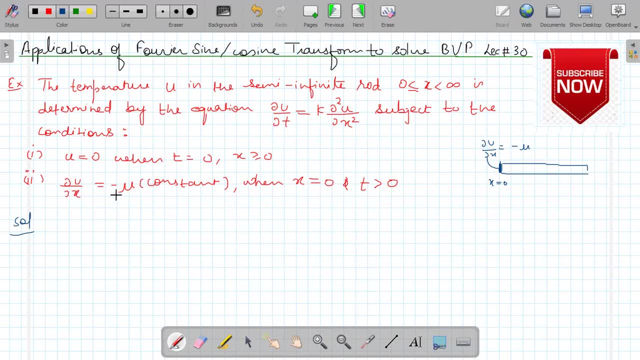 del u by del x is equal to minus mu. so we apply here Fourier cosine transform, as I have discussed in my lecture number 29. so whenever we are given derivative condition, we apply Fourier cosine transform. so we apply Fourier cosine transform on the given equation del u by del t. 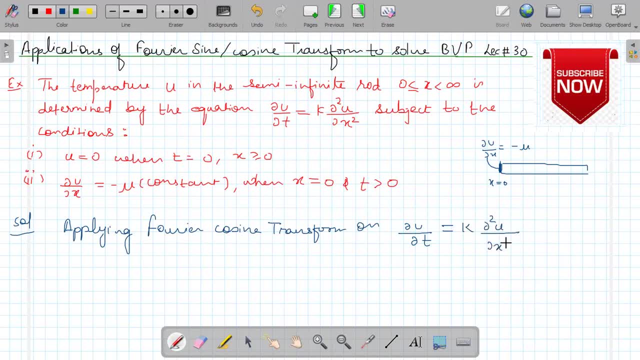 k del 2 u over del x square. so Fourier cosine transform is zero to infinity del u by del t cos px dx is equal to integration. zero to infinity k del 2 u over del x square cos px dx by the definition of Fourier cosine transform. okay. 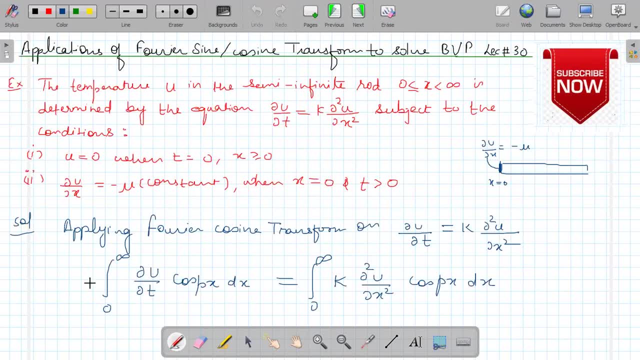 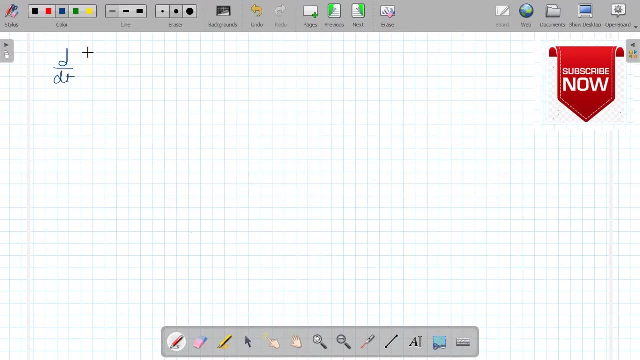 now, as you can see, this integral is with respect to x, so we can take this derivative outside in the form of D over DT, D over DT, zero to infinity, u, x, t, cos, px, dx, and on the right hand side we can take k on our outside the integration, and then we integrate that. 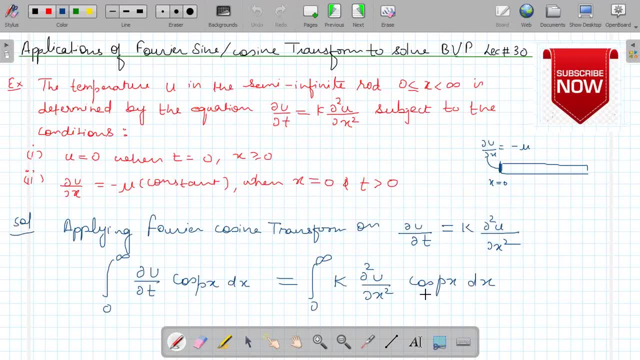 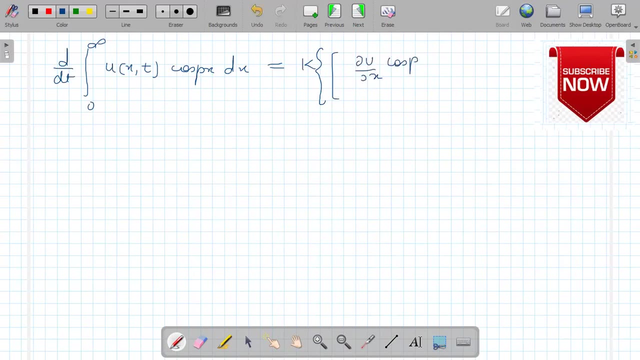 so it is our first function and this is our second function. so we have first function into integration of second function. so we have del u by del x cos px, zero to infinity limit on this minus del u by del x cos px. this minus integration del u by del x and differentiation of this. 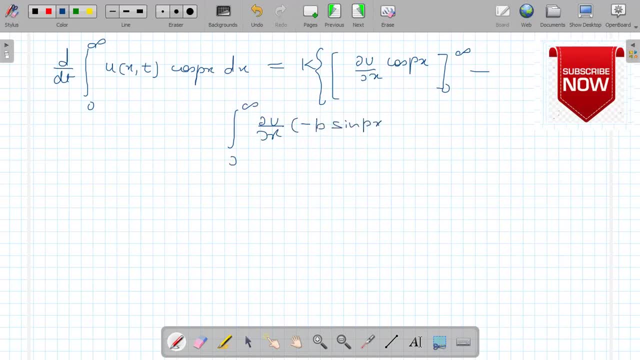 minus p, sin px, dx. okay, this whole expression can be denoted by U C bar. so we can write this as D U C bar over D T minus K, because at upper limit this is zero. at lower limit this will be del U by del X at the value at del U by del X at the point 0 comma T. 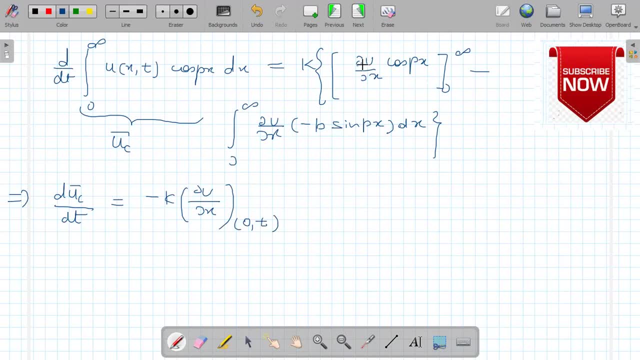 okay, because U is a function of X comma T, so del U over del X is also a function of X comma T. so at lower limit means the value of del U by del X at X is equal to 0 comma T plus. because of this negative sign and this negative sign we have positive sign. 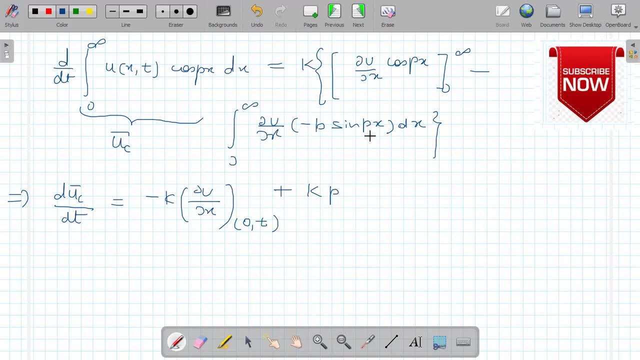 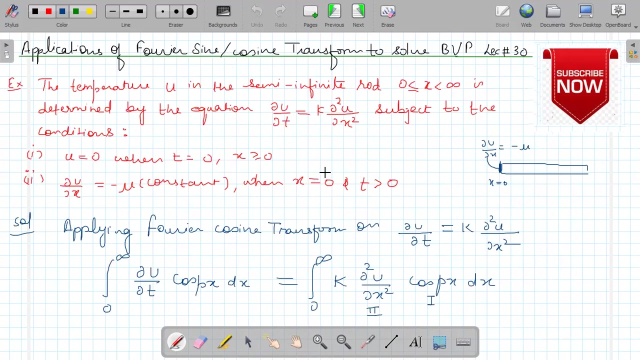 K into P. this K will multiplied with this expression also and we have integration del U by del X into sine of P, X, D, X. so we have D U, C, bar over D, T is equal to K. this is given to you as del U by del X, as minus mu, when X is equal to zero and T is greater than zero. so we can replace Hu by applies. 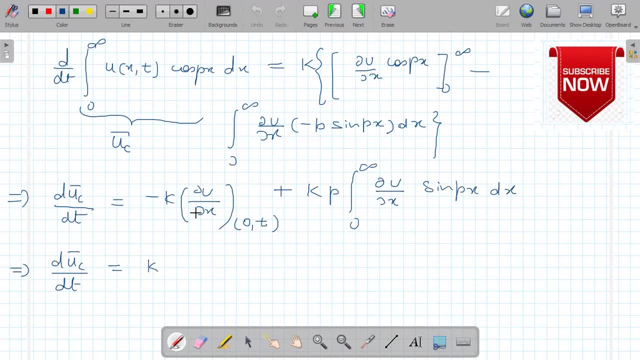 som and T is greater than zero, and T is greater than zero. so we can repeat the 1 with P, P. we can replace this by minus mu. So when we replace this by minus mu, this minus and this minus will make positive sign here and we have only mu plus kp. We again take this. 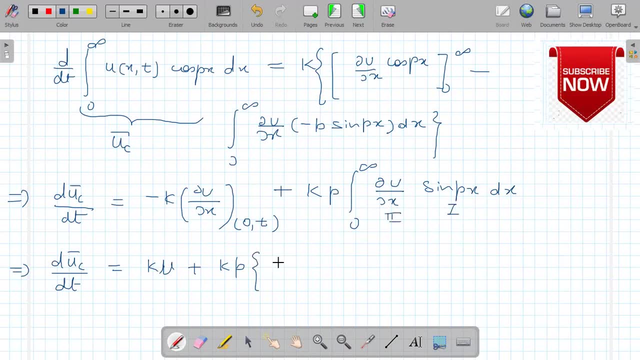 as first function and this as second function. So we have ux t, sin of px. first function. integration of this will be u, limit zero to infinity. then integration ux t and differentiation of sin is p, cos, px, dx. Okay, k, mu plus at upper limit this will be 0, because we suppose that as x approaches infinity, u. 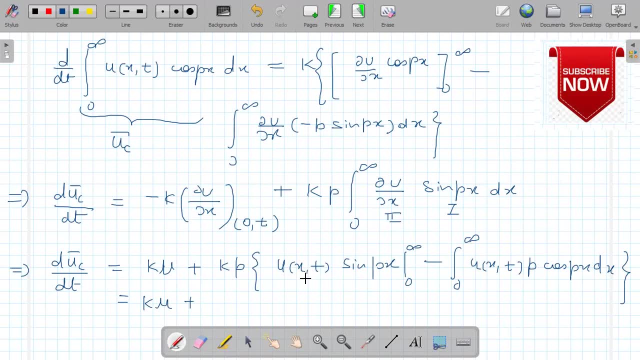 approaches to 0, okay, and at lower limit, this will be automatically 0. so we have this expression only. so we have 0. this is when you take p outside. this will be 0 to infinity. u, x, comma, t, cos, p x, dx. so this is nothing but. 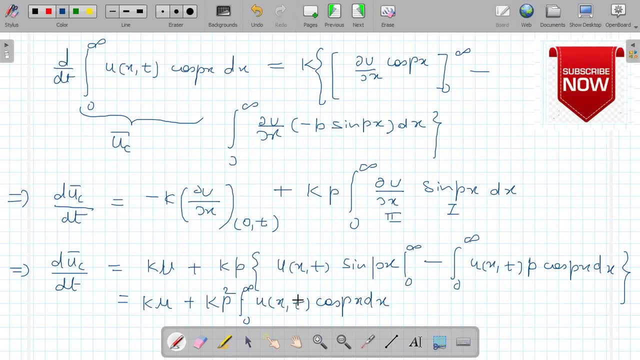 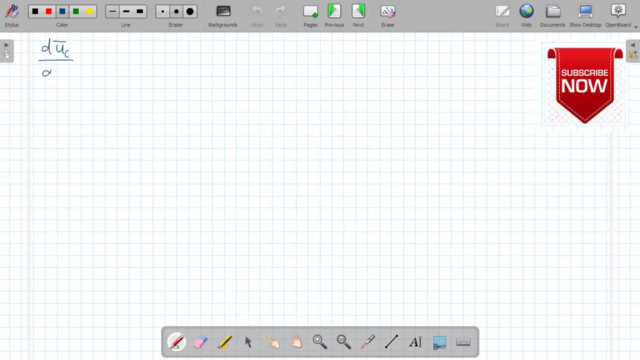 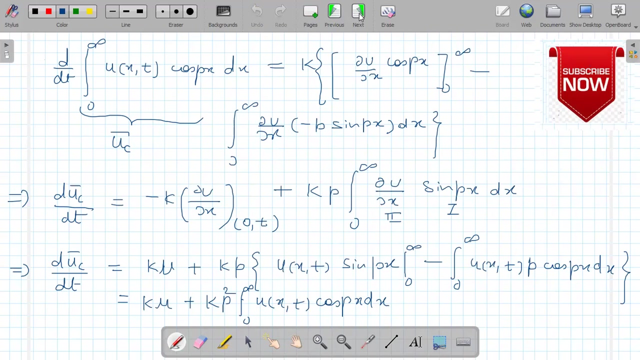 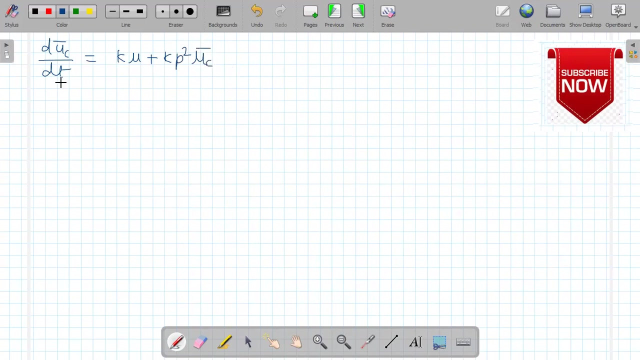 fourier cosine transform of the function u. so this integration can be replaced by u bar, u c bar. okay, so we can write d u c bar over d t, k mu plus k p square mu c bar. so we have this differential equation which you arrange. you will get d u c bar over dt minus k p square u c bar, k mu. So this is a linear differential. 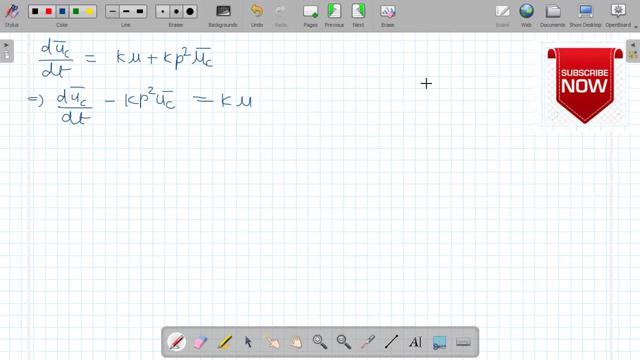 equation whose general form is: dy over dx plus py is equal to q, where p and q are the functions of x. So we have: in place of y, we have u, c bar. in place of x we have t, and this is p, and here k, mu is q, and both are constants. They may be constants also, So we will find. 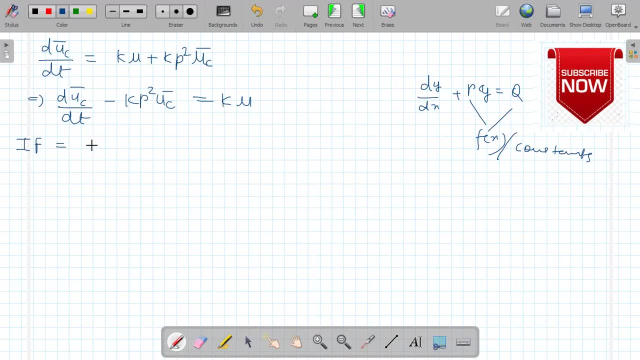 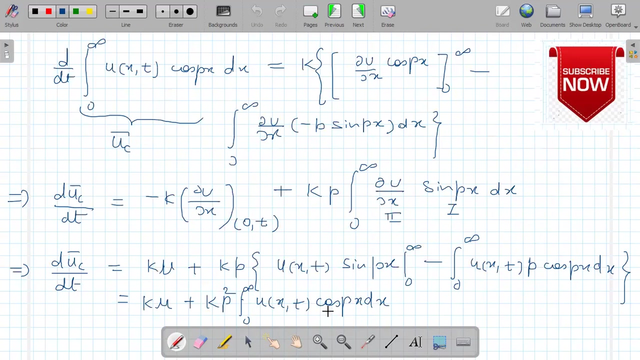 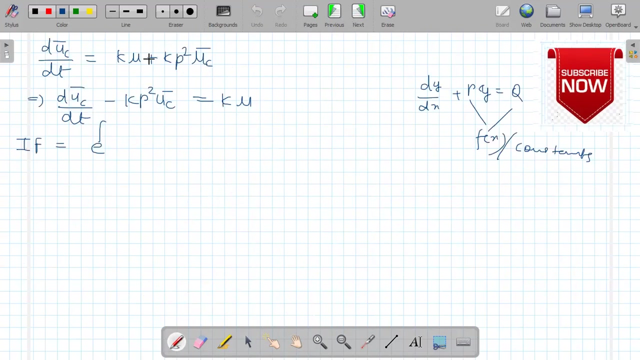 the integrating factor. Integrating factor is e raised to the power. Here we have negative sign. Let me make a correction. So here we have negative sign Minus k p square u c bar, So that we have positive sign here. So k p square dt. Okay. 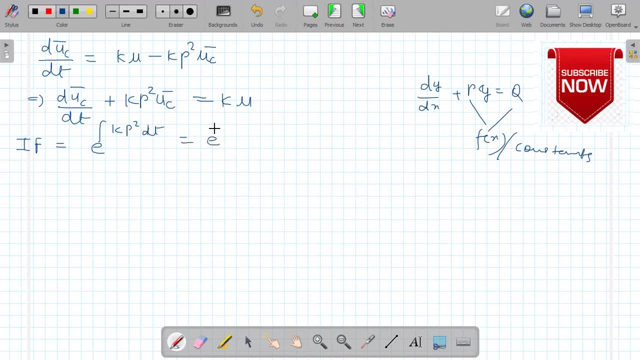 And this value is e raised to the power k, p square t. So the solution of above equation is linear. So here differential equation is integrating factor into u c bar, Since u c bar is the function of p t because it is a Fourier transformed functionva after four years of. 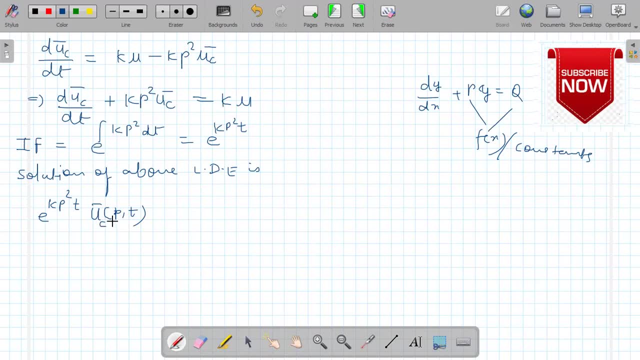 I actually, of course, translated it into unexpected nowadays, actually two years old, and now I am reading myfield. So I am calculating the for taking the Fourier transform, cosine or sine transform, we always get the function of P. that's why X is replaced by P here, and integration Q, which is K, into mu. this is Q. 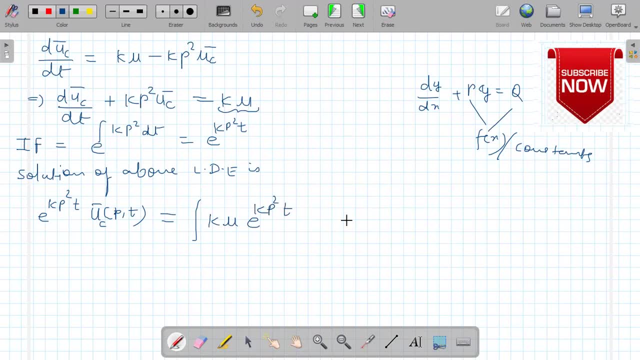 and integrating factor is K P square T, DT plus C. K, mu, e raise power. K P square T whole divided by K P square plus C. so the value of mu, C, P comma T is mu over P square. this exponential will cancel with this and plus C with. 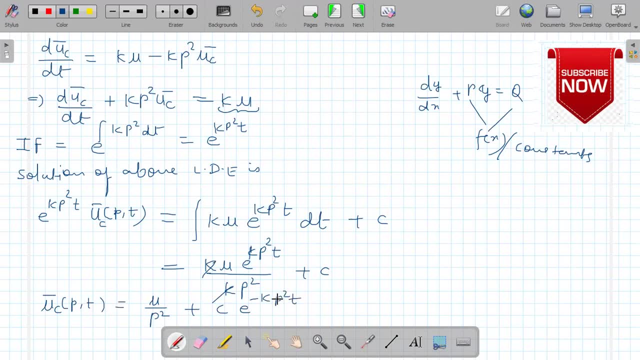 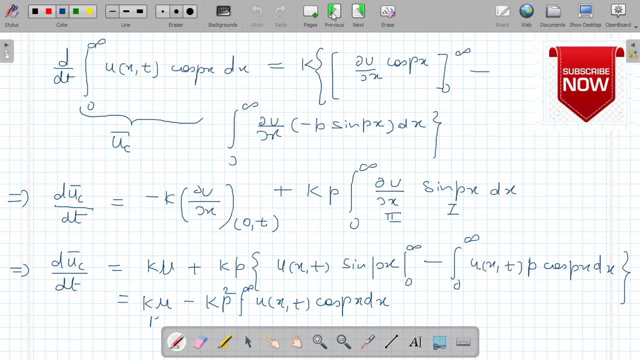 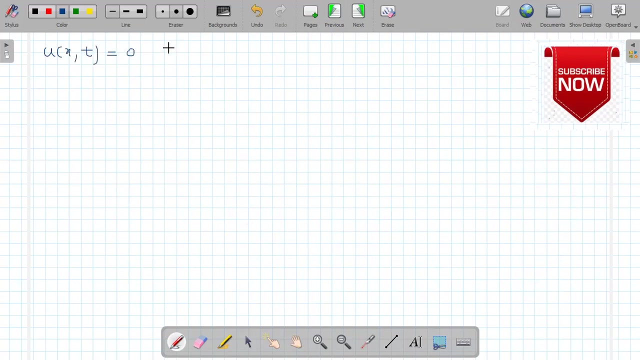 multiplied with minus K, P square T. mark this as equation number one. now we need to find the constant value C. for that we use this condition. okay, we are given that U is equal to zero when T is equal to zero means U X comma T is zero when T is equal to zero. so you have U C bar P comma T. so what we will do is take: 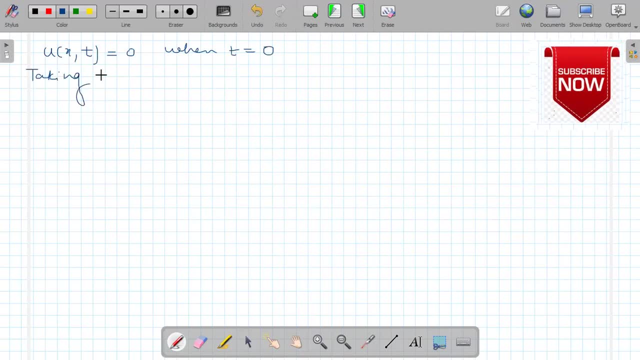 its Fourier cosine transform, for the Fourier cosine transform of this equation, this condition, basically. so we have integration: zero to infinity. U, X, comma, T cos, P, X, D, X, ok is equal to zero. We put t is equal to zero. you replace t by zero here, u, so that we need 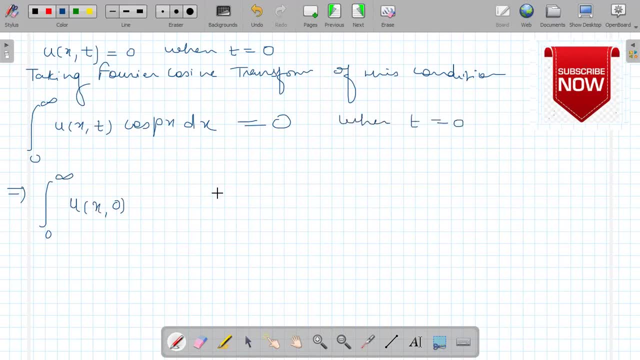 not to write again and again when t is equal to zero. So we have done this, we have replaced t by zero. Now this is. this whole can be represented by u, c, bar, p, comma zero, and this is equal to zero. So we have this condition. So, substituting this condition, this condition, 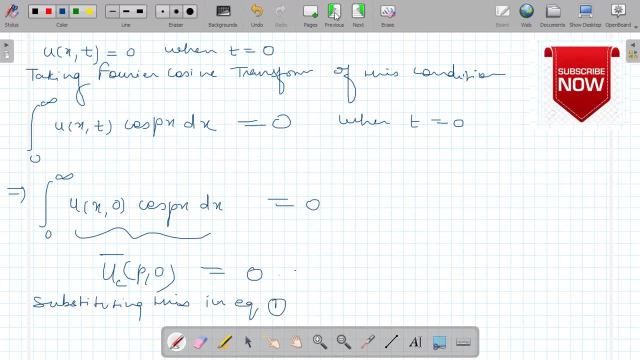 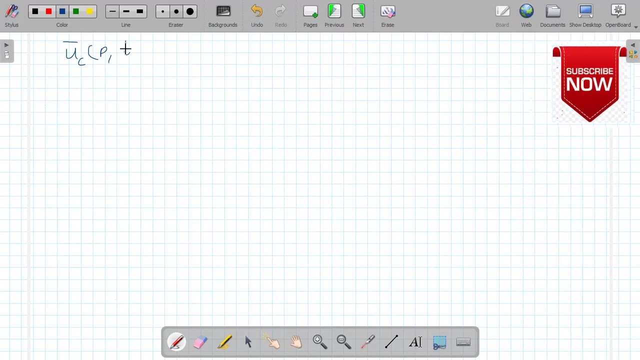 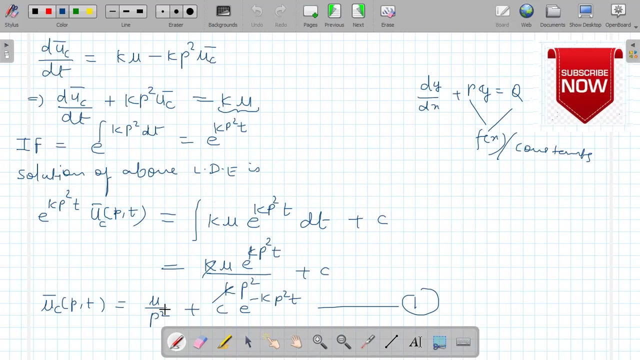 this in equation one. What is equation one? u c p, t is equal to this. So we put u c bar p. we put t is equal to zero there, So that we have on the right hand side we have only mu upon p square plus c. 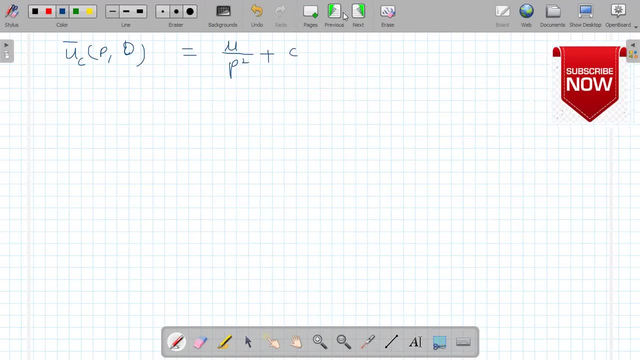 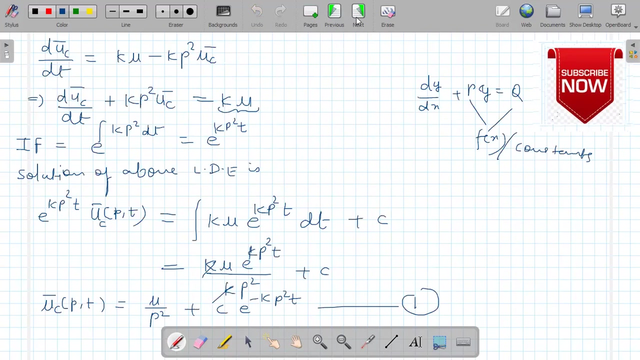 So and this is equal to zero. because of this condition, u c bar p, zero is zero. So we put is equal to zero, So that the value of c is p square, Its value will be here. Now this value we can substitute in this equation, in equation number one, So from equation one: 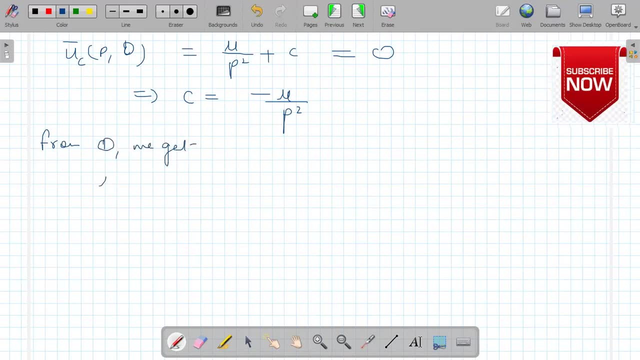 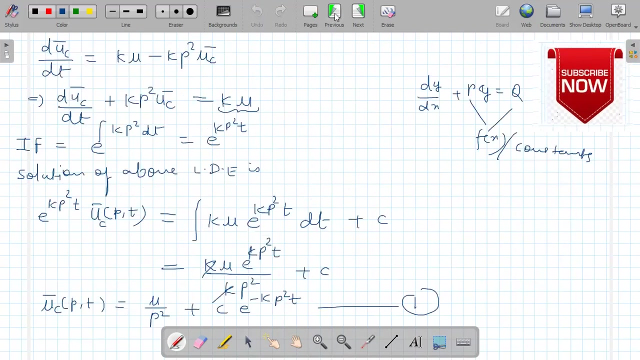 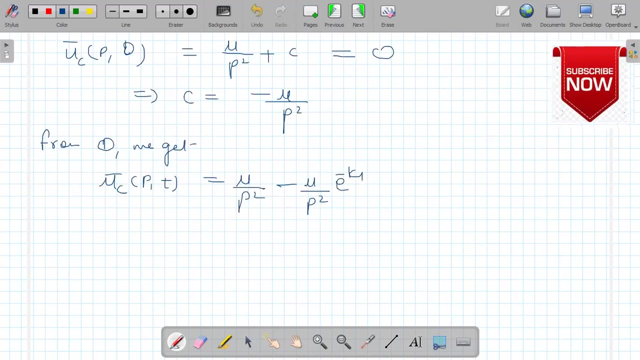 mu c bar p comma t is equal to mu upon p square plus c ki jaga is ki value substitute karenge. so we use the negative sign mu upon p square and a to the power minus k p square t, so we can take mu upon p square common. we have this now. this is the value of mu c bar, which is: 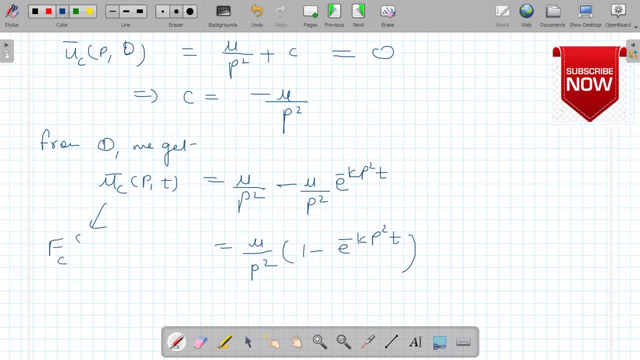 the four year cosine transform of u x comma t. to find u x comma t we need to take four year cosine inverse of this. so u x comma t is four year cosine inverse of this function, which is the function of p. so okay, so by definition of inverse four year transform, it is equal to two upon pi zero, to infinity, nu upon. 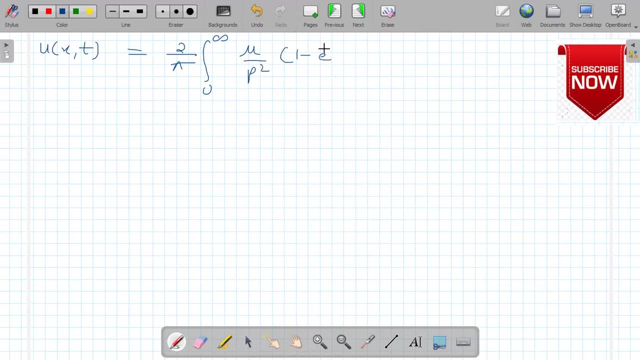 p square into one minus a to the power minus k. p square t. p square t into 1 minus k на mu c. k to cos px dp. Generally when we take Fourier cosine inverse transform or sine inverse transform, we always get some complicated expression inside the integration. You can see here that 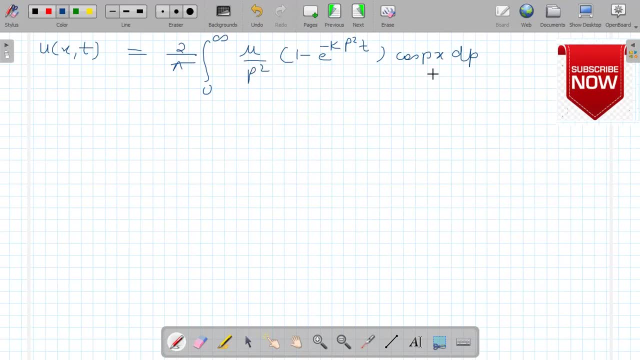 both of these. we have functions of p and doing the integration of this expression is not so easy. So generally we leave such expressions as it is, by taking constant terms outside the integration if it is applicable. So we leave this expression as it is, by taking 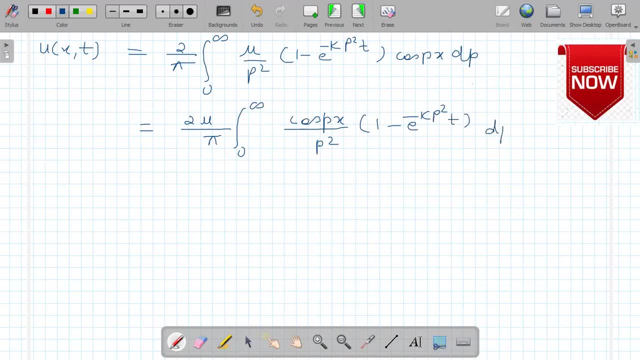 constant terms as it is, and this will be the answer for the given problem. Okay, So now let's do the second example. Solve del U by del t is equal to the square root of px del two u over del x square. where x is greater than zero, t is greater than zero, such that: 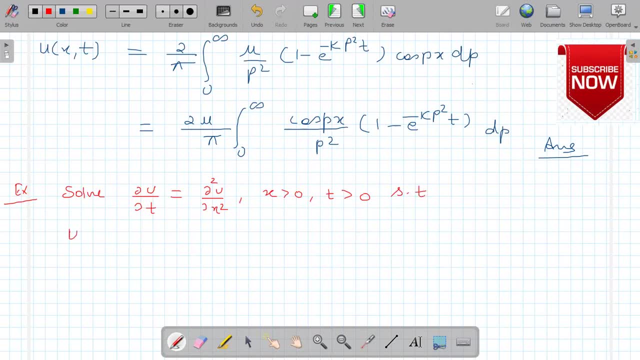 we have u x zero, comma t is equal to zero and u x comma t is bounded and u x comma zero is x for x line between zero to l and zero for x line between zero to l and zero for x line between zero to l and zero for x greater than l. 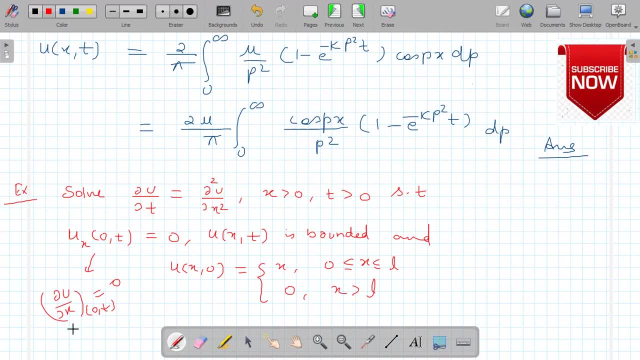 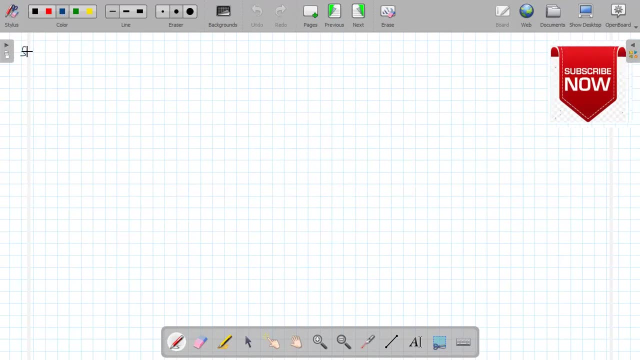 so we are given the derivative, so we are given the derivative condition, so we apply fourier cosine condition, so we apply fourier cosine transform over this. Applying Fourier cosine transform on del u by del t, del 2 u over del x square, We get 0 to infinity del u by del t, cos px. 0 to infinity del 2 u over del x square, cos px dx. 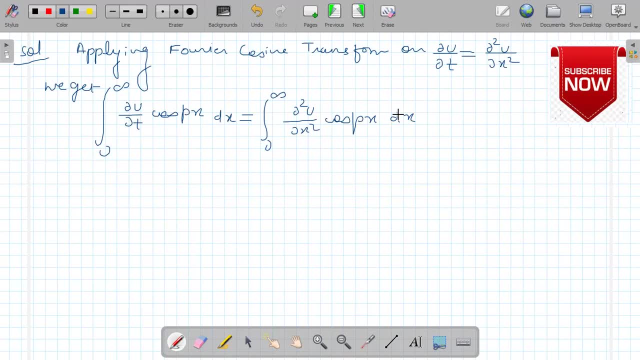 Again, we take this del over dt outside, so that we have d over dt of integral u cos px dx. And here we have del u by del x cos px, minus del u by del x p sin px dx. This is nothing but d? u c bar over dt. 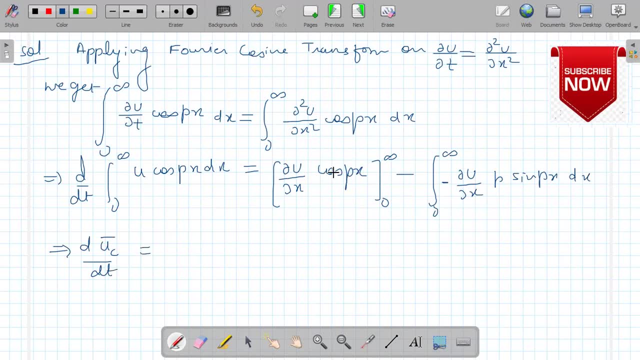 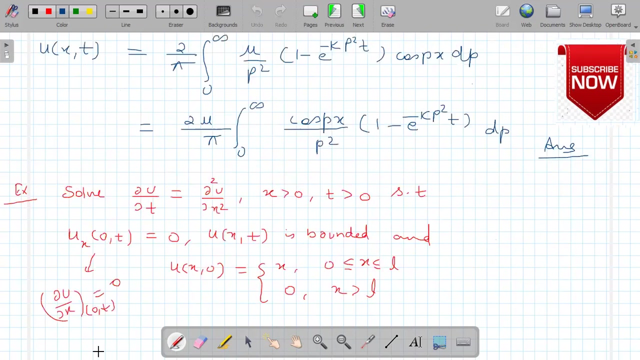 This is 0 at upper limit and at lower limit This is minus del u by del x At 0 comma t. plus again, We integrate this 0 to infinity del u by del x, sin px, dx. We are given the derivative condition del u by del x at 0 comma. t is 0.. 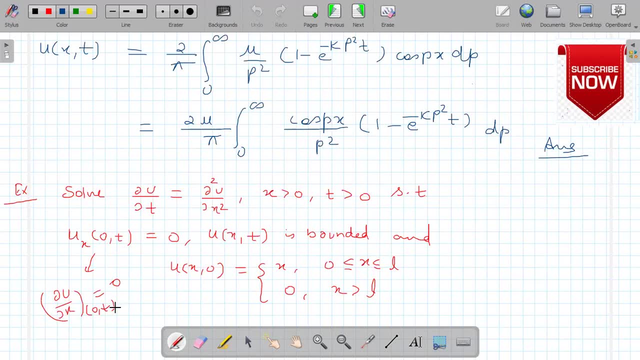 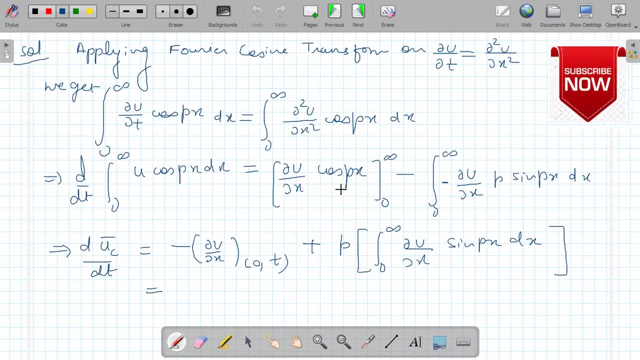 Okay, And also you should write that we are assuming that del u by del x approaches to 0 as x approaches to infinity. You should write this somewhere. Okay, don't write it directly, Otherwise it will make confusion. So I should write here: 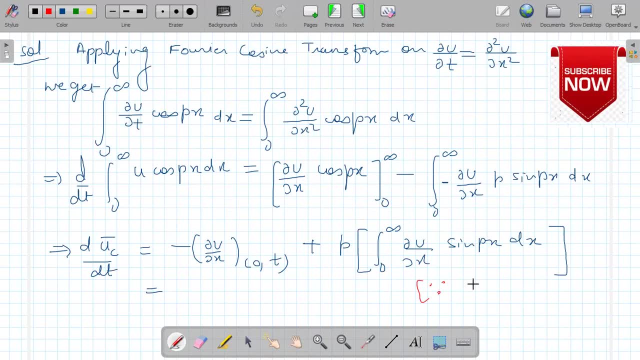 Since We assume that del u by del x approaches to 0 as x approaches to infinity. Okay, Okay, So this is 0, because we are given that this value is 0.. So we have 0 plus this, So we solve this. 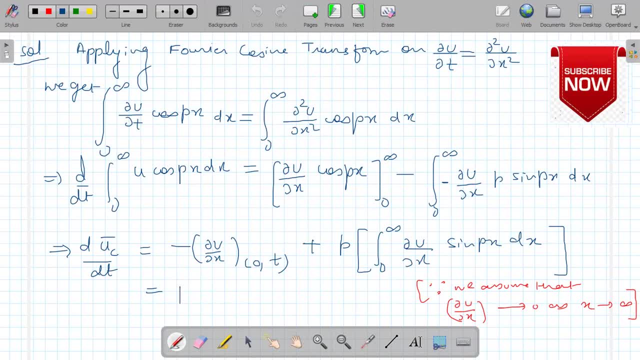 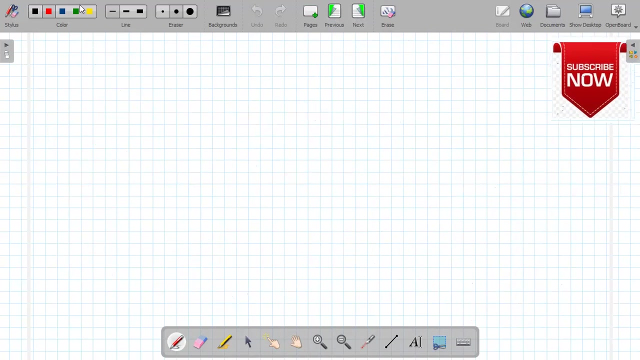 Now this is equal to p integral 0 to infinity. del u by del x sin px dx. Okay, Here we also write the reason for this, because del u by del x is 0 at x is equal to 0.. We have d u c bar over d t. 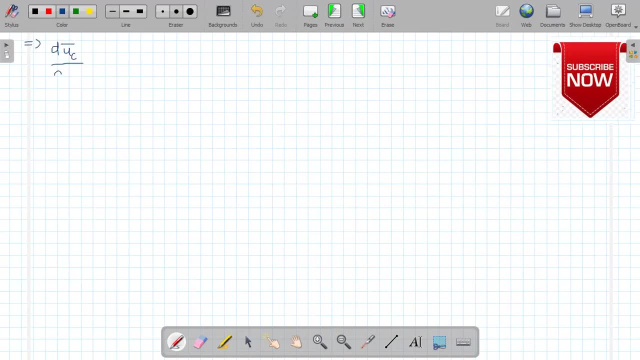 Is equal to p. p? u sin px minus p? u cos px dx. Again, Assuming that u approaches to 0 as x approaches to infinity. Okay, So this is 0.. So we have d? u c bar over d t. 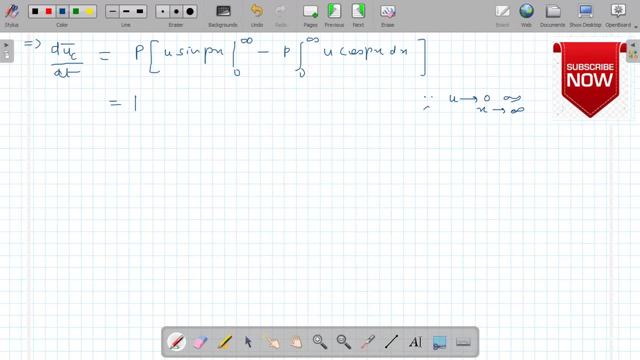 And at lower limit, this will be 0.. And we have p square. This is nothing but u c bar. Okay, This expression vanishes. This is 0.. And we have d u c bar over u c bar, So we can do something with this. 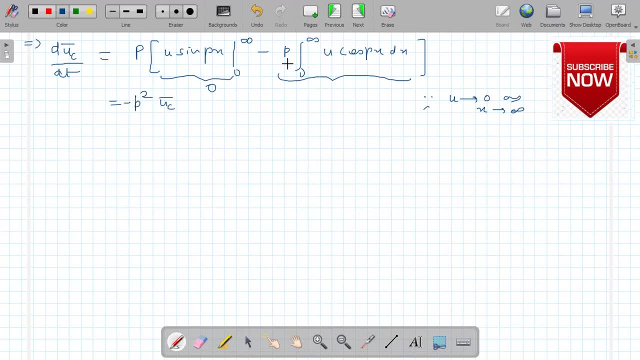 Where p into p is p square, And this integration of u cos px is denoted by: Does the Fourier cosine transform of the function u? Short form is u c bar. Okay, So we have d u c bar Over u c bar. 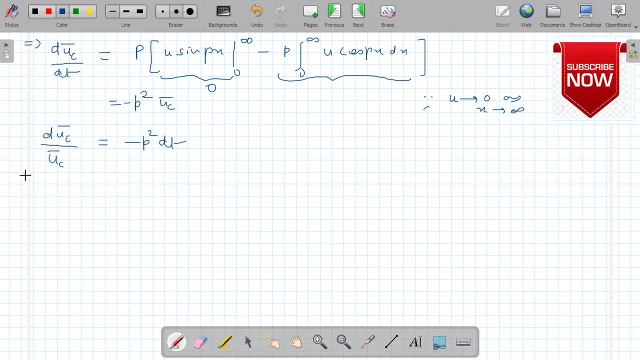 We can separate the variables, The variables separable differential equation, integration. Integrating this, this is variable, separable differential equation. So integrating it, we get log of uc bar minus p, square t plus log of c, So that we have uc bar, log of uc. 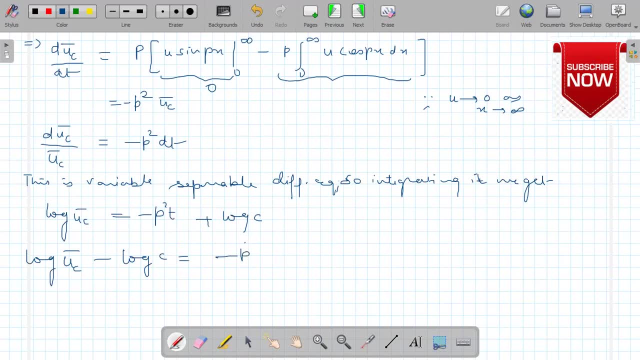 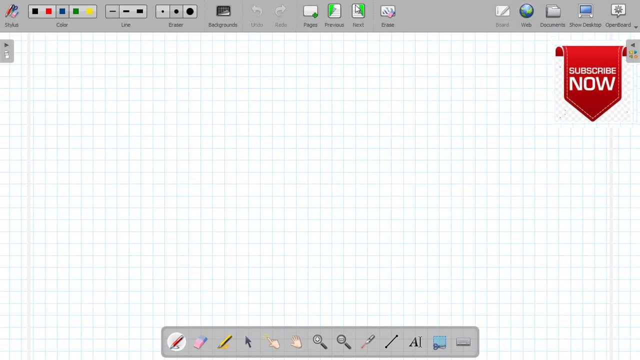 bar minus log of c. So log of uc bar over c. This implies uc bar over c is equal to e to the power minus p square t. This implies uc bar is equal to c to the power minus p square. So log of T. now we write it in this form. so to find the value of C we put T is equal to. 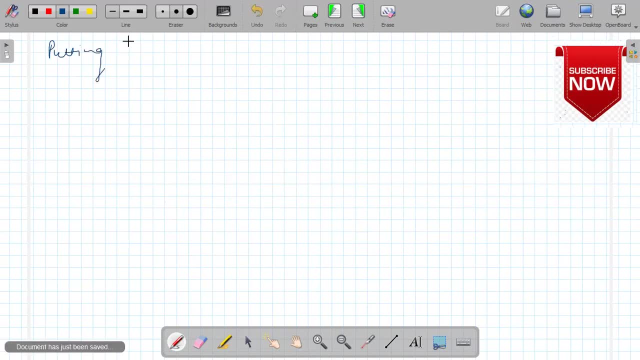 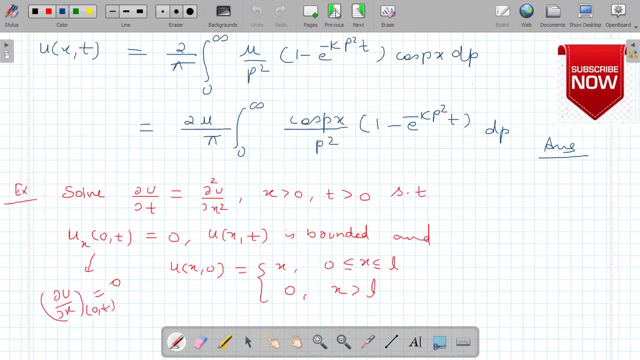 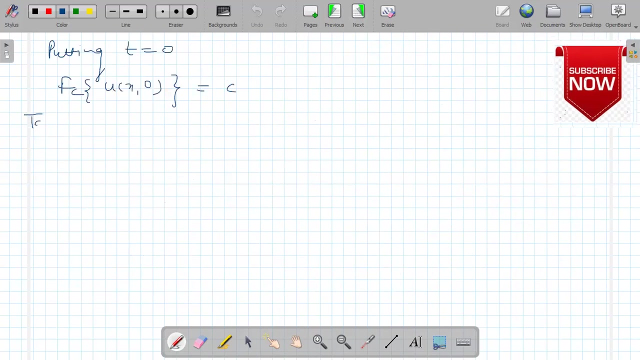 zero, we get Fourier sine transform of ux comma zero is equal to C. you are given this condition in the question. this one ux comma zero is x, so we will take the Fourier cosine transform of this condition. okay, taking, let me write the expression first, since ux comma zero is x or x, lying between 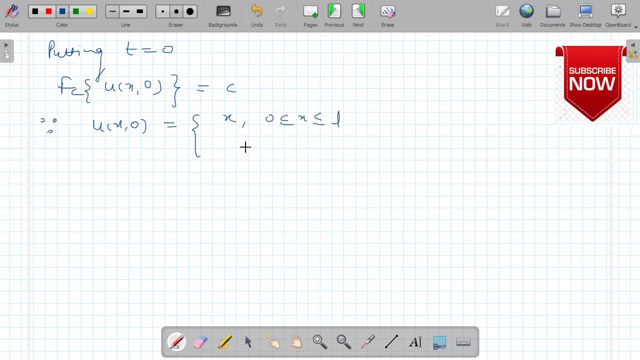 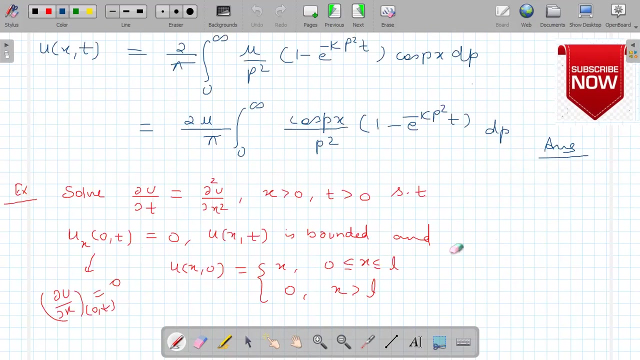 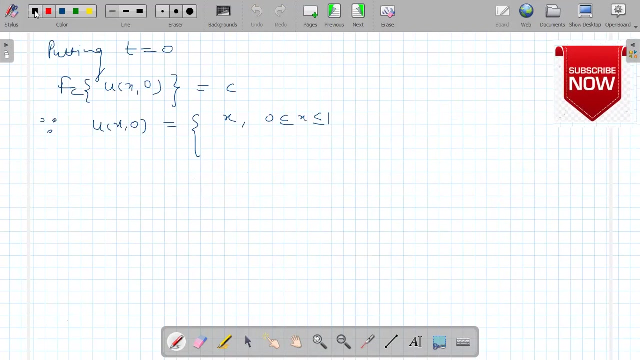 zero to L. for simplification, let's replace L by one. okay, let us replace this by one. so. and zero for x greater than one. so, taking Fourier sine transform of ux comma zero is equal to C cosine transform of this condition, we get integration zero to infinity. ux comma zero, cos PX, DX is equal to we split this limit. 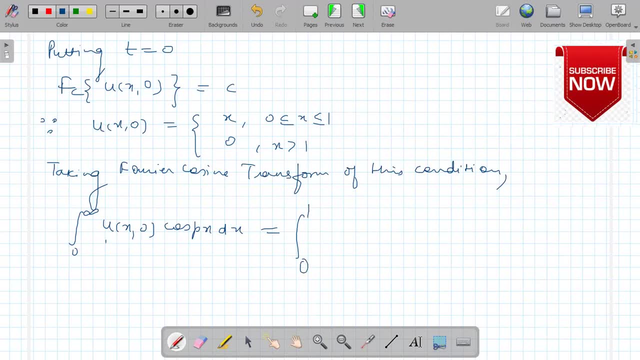 into 0 to 1 and replace ux0 by x cos px, and for 1 to infinity, we have 0 cos px, px. So this expression is 0.. When you solve this, you will get first function, integration of second function, which is sin px over p, and then we have minus sign, differentiation of. 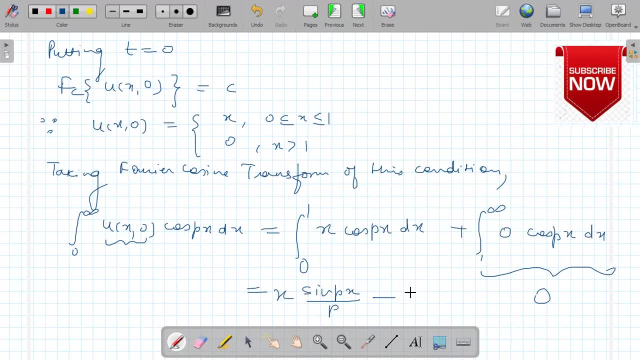 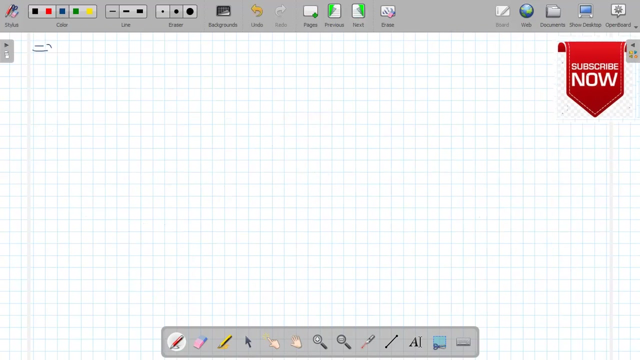 this and integration of this again, which is negative. so we have positive sign cos px over p square, Applying the limit 0 to 1, so that we have sin px over p. This left hand side is denoted by fc of ux, comma 0. So we have fc ux comma. 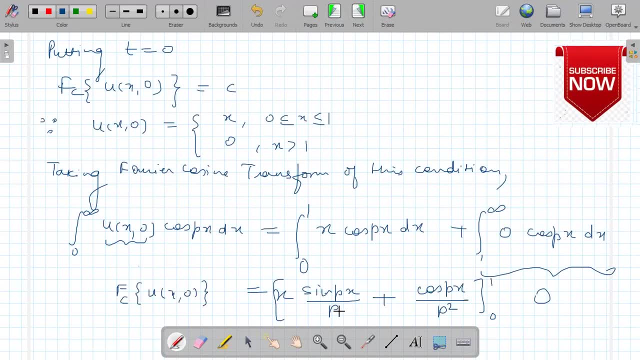 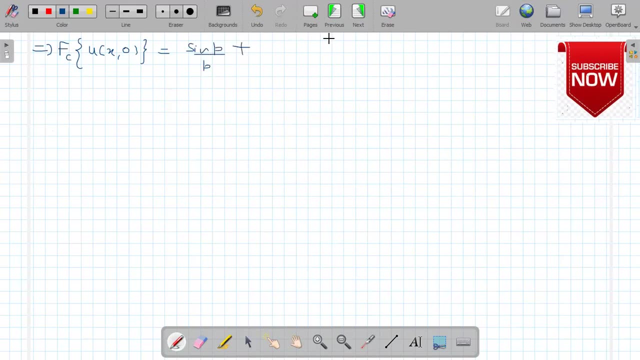 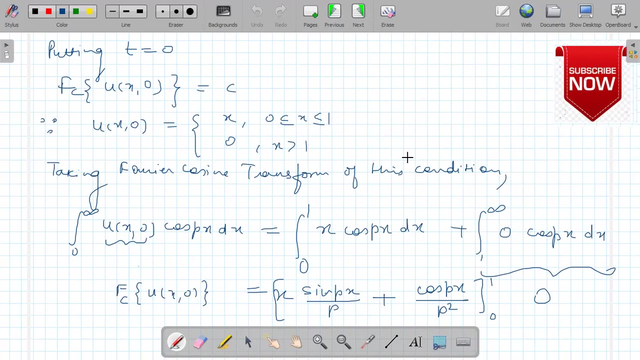 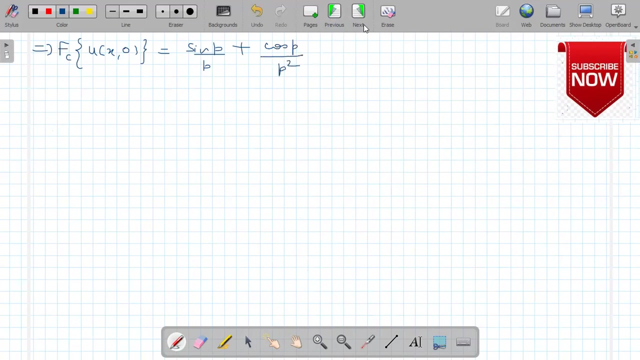 0 is equal to sin px over p. Ok, So we have sin px over p. So this left hand side is denoted by fc of ux, comma 0.. So we have sin px over p plus cos px over p square, Cos px over p square At lower limit. this will: 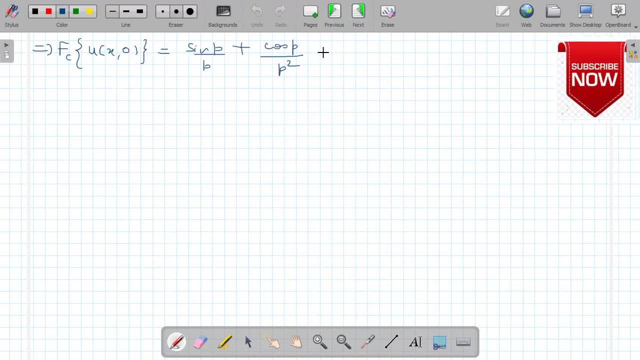 be 0 and this will be minus 1 upon p square. So we have sin px over p plus sin px over p. So we have sin px over p x- Sorry, plus cos px minus 1 over p square. So we come to this condition. We have obtained a. 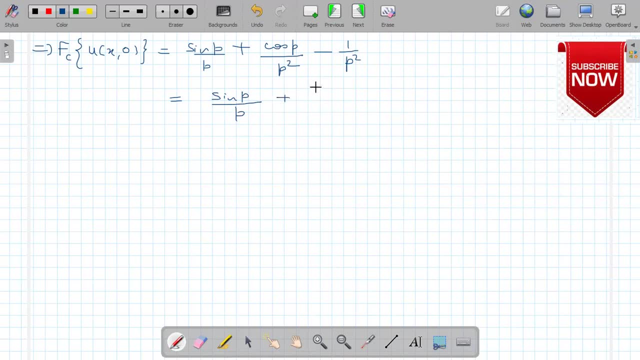 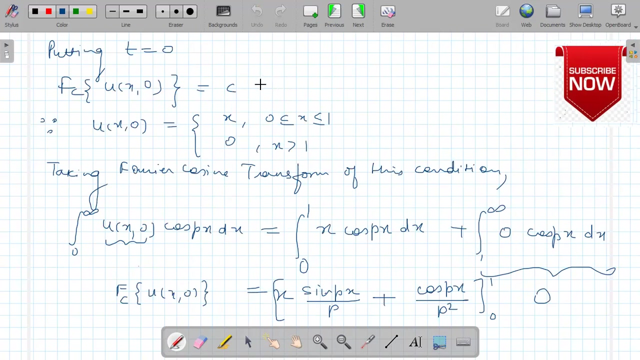 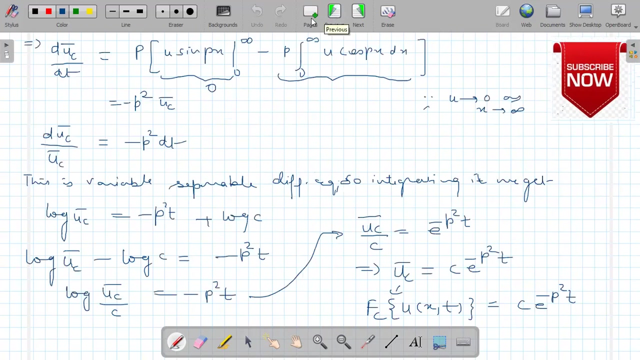 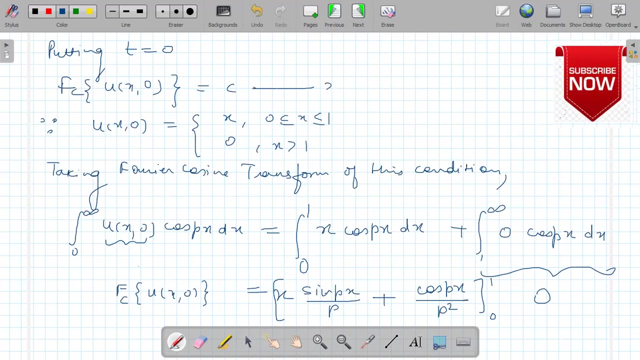 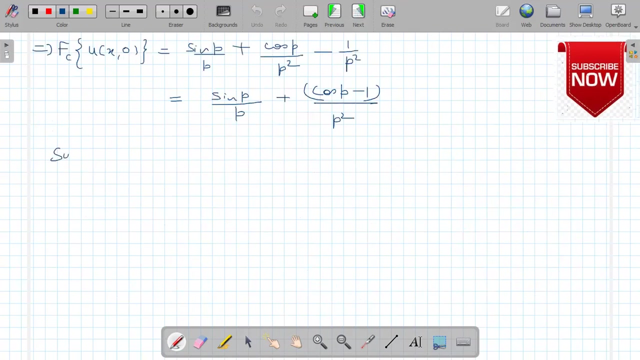 So we have sin px over p x Sorry- plus cos px over p, plus sin px over p square. So we come to this condition. We have obtained a, this solution. this is the value of C that we obtain from equation number two. we're taking value of f in equation number. this is equation number two. 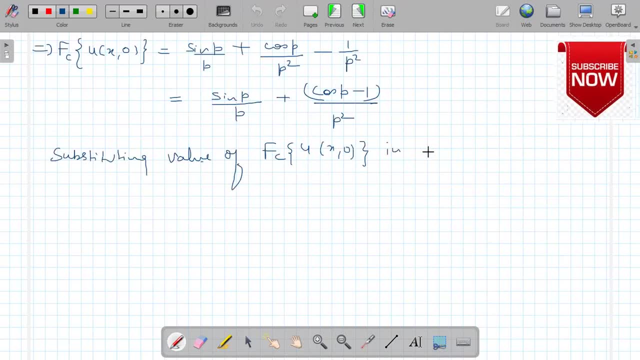 where we substitute this value, so we receive value of C, we get C is equal to P plus cos, P minus 1 over P square. okay, now substituting the value of C in equation number one, we get value of Fourier cosine transform of u X comma T. 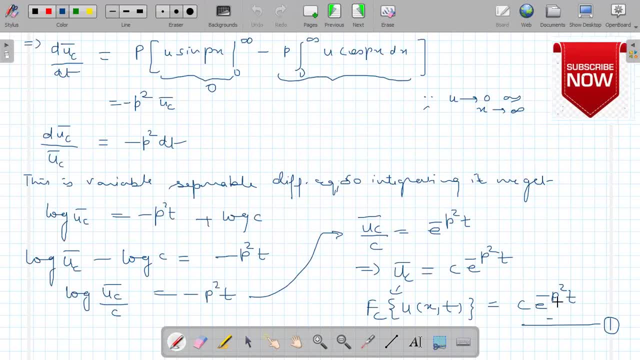 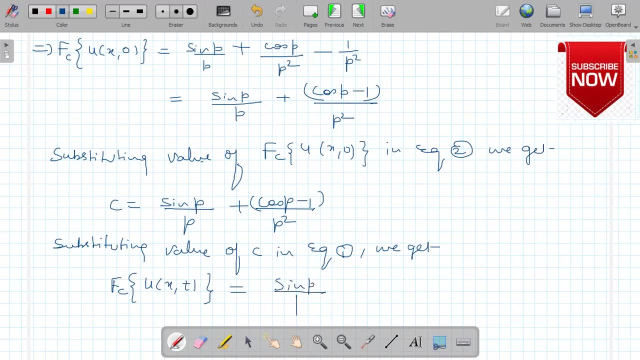 this is equation number one. this one is equal to sine P over P plus cos P minus 1 over P. square into E: raise power minus P square T. now we'll take the Fourier cosine inverse of this whole expression to get the value of u X comma T. okay, u X comma T is nothing but Fourier cosin inverse of Fourier. 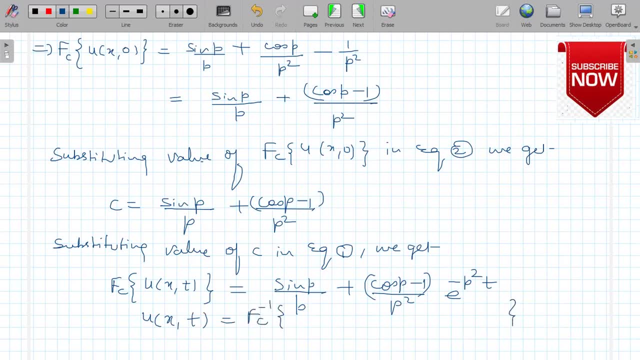 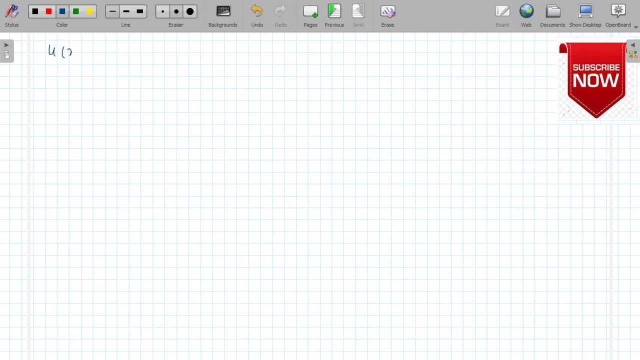 cosine inverse of this whole expression. okay, so the ux comma T is 2 upon pi, integral 0 to infinity, sine P over P plus cos P minus 1 over P square e raised power minus P square T, cos Px dP. we leave it here. this is the answer because 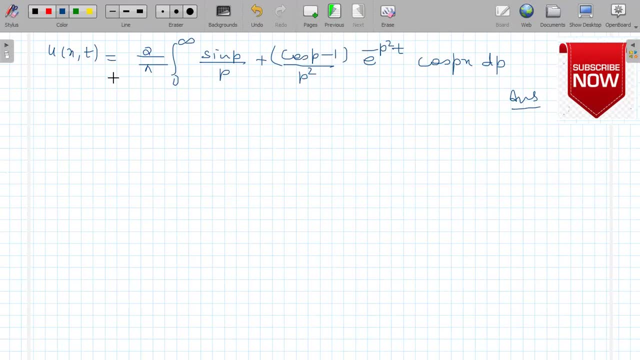 it can't be solved further. it is very difficult to solve it, so we generally leave at this point after taking the inverse transform. okay, okay, so I hope you understand both examples and the reason behind why we are applying Fourier cosine transform in these two questions. okay, so you can try.